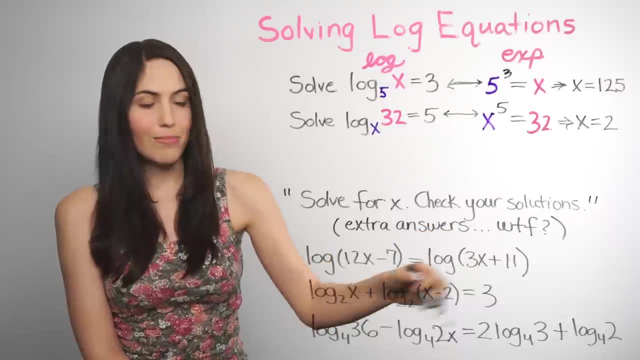 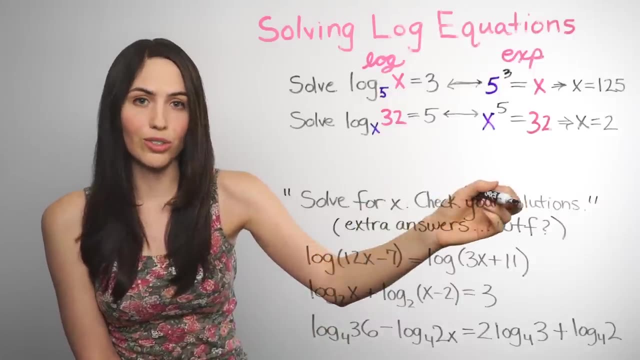 equals another log. Several logs equals a number, Many logs, Some with numbers multiplied out front. What do you do? And what do you do if you see something like check your solutions, or if your teacher says: check for extraneous solutions or check your answers? 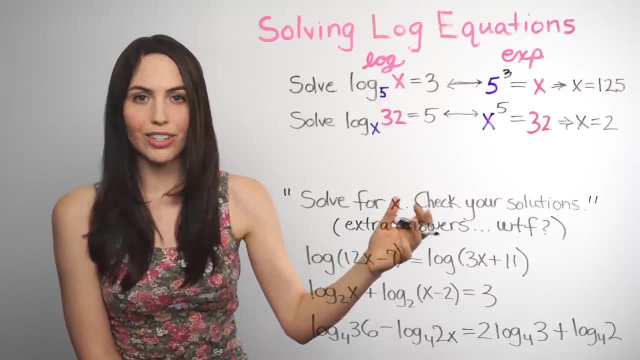 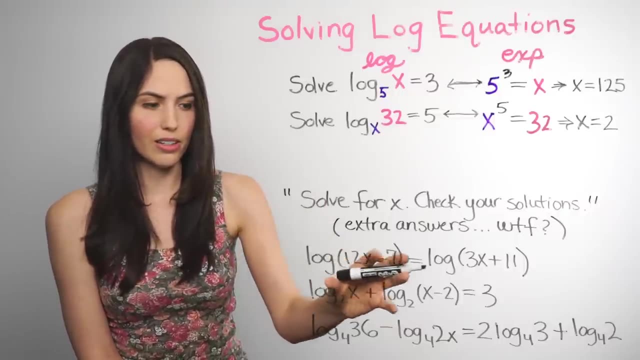 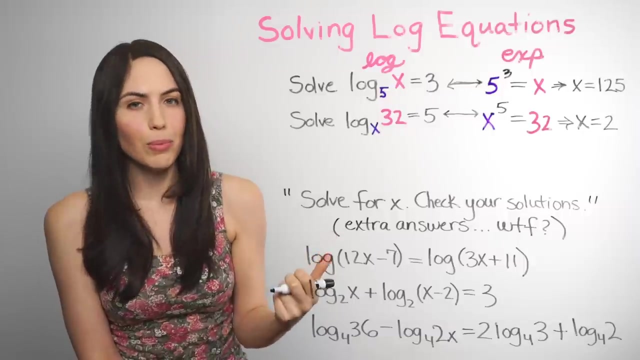 Check for extraneous solutions or check your answers. to do that, I'll show you and also show you the log properties, which are what you need to simplify and condense and solve more complicated equations like that. so that would be like the power property, quotient property, product. 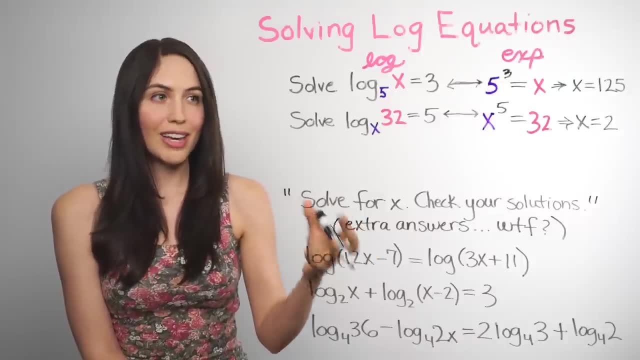 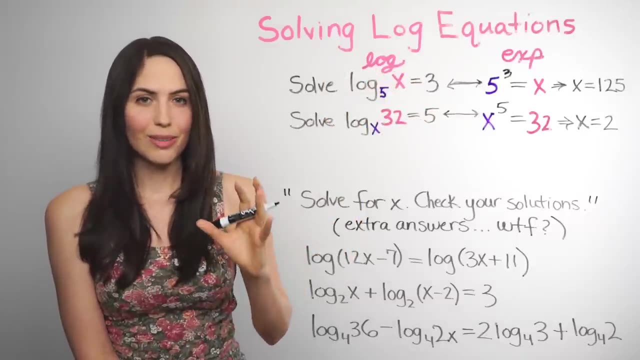 property, equality property, all of those. so my other video gave you a taste of solving log equations at the end, and now I'm going to give you a whole meal, but if you see the kind that you're working on, you can skip ahead. so just check the. 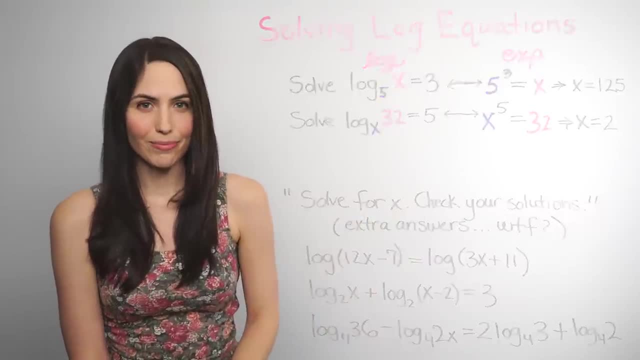 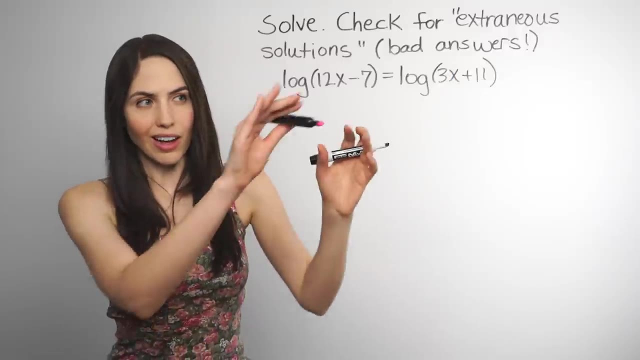 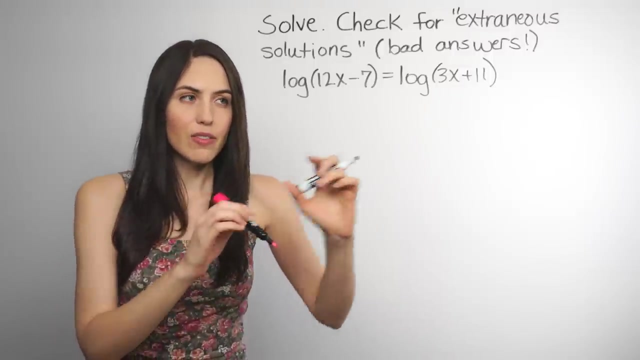 description for the time to jump to. let me show you how to solve. all right, say you have a log on each side of the equation. it's getting more complicated, but don't worry, don't panic, because actually really simple. if the logs have the same base, you can just set the insides of the logs equal to each other. 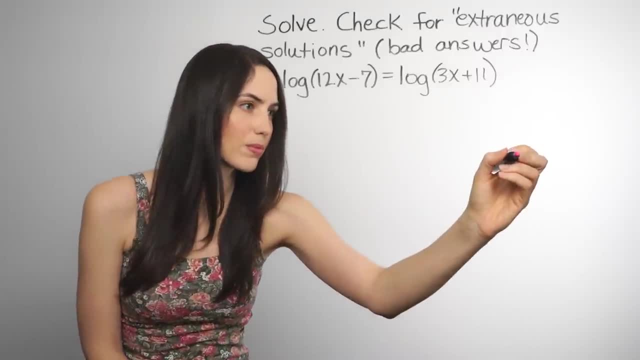 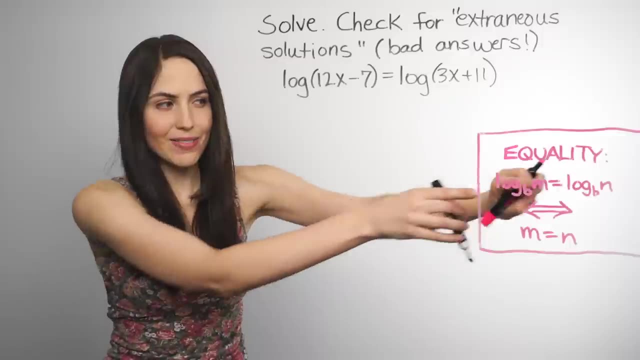 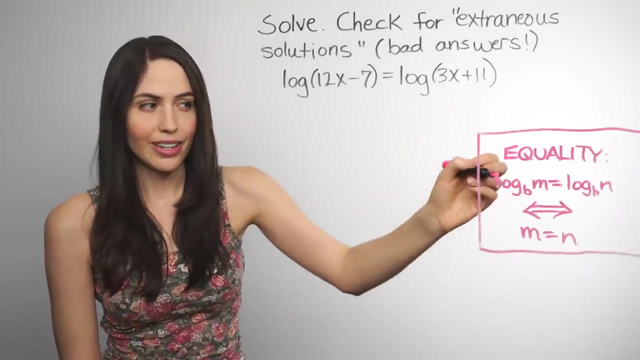 and solve. so this is the equality property and it's just like I was saying, if the little bases are the same, you can take the insides of the log and set them equal to each other. by the way, this is for little bases that are positive and 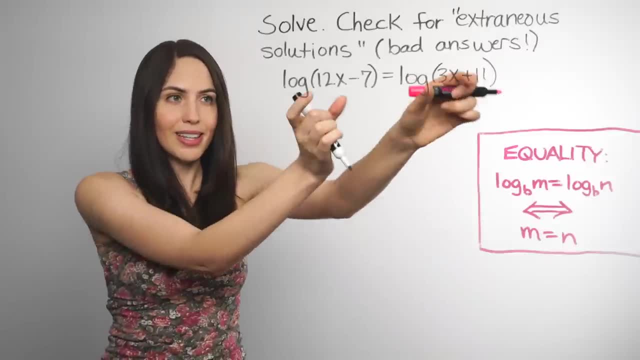 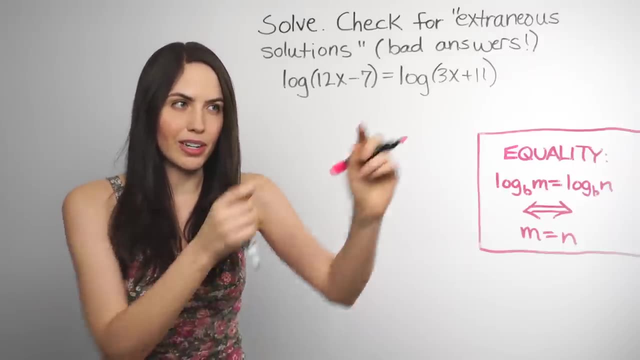 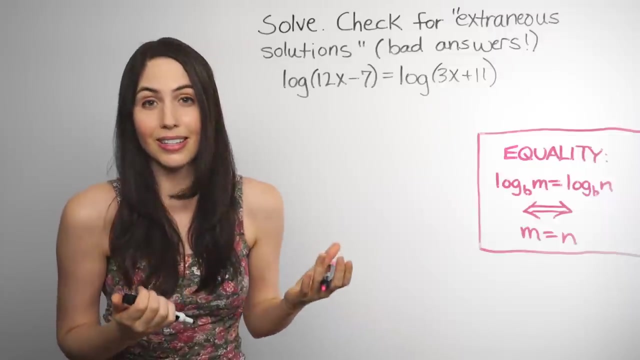 not equal to one. but anyway, if the bases are the same, you can set the insides equal. and I know what you're thinking. what bases? I don't see any faces. yeah, they're not explicitly written here. if you don't actually see them, it's implied to be 10, the common log. so that's like the default and we can just. 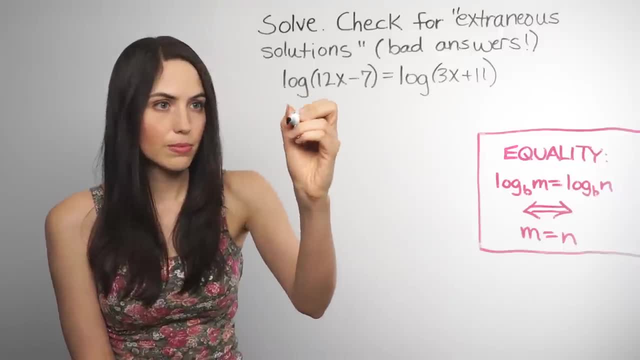 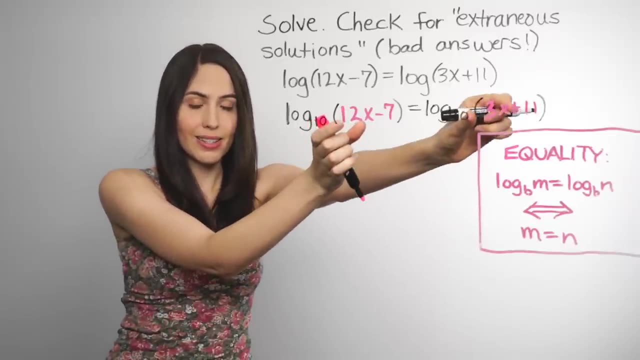 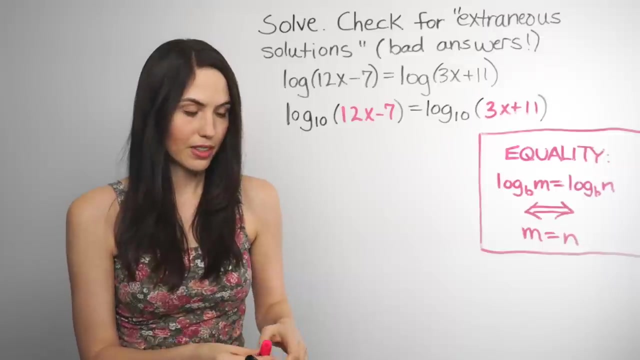 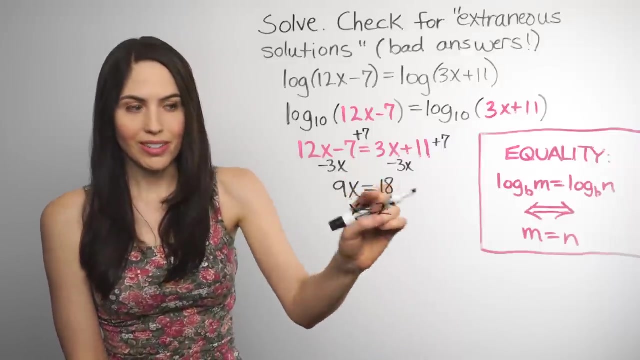 go ahead and write that and now that we can see that those spaces are actually the same, you really do. just take the inside x expressions, set them equal to each other in a new equation and leave the logs behind you, you, you, some algebra and solve: You get x equals 2. And I know you might think that you're. 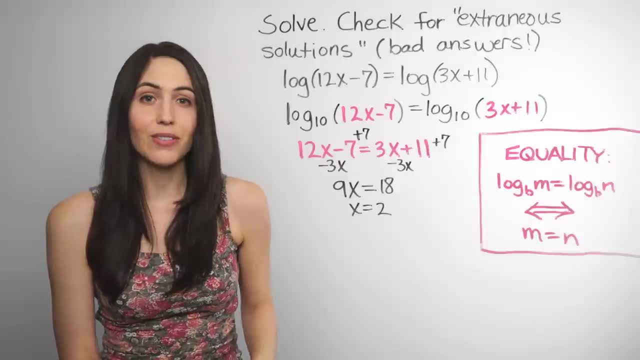 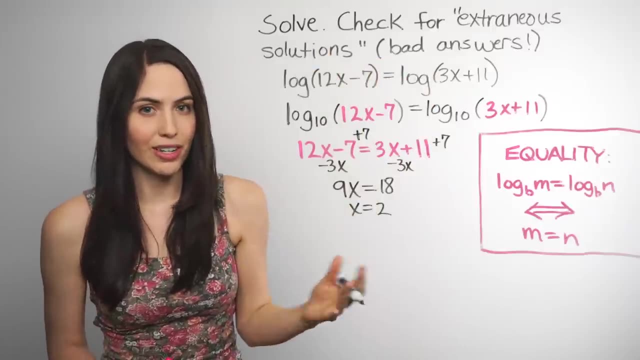 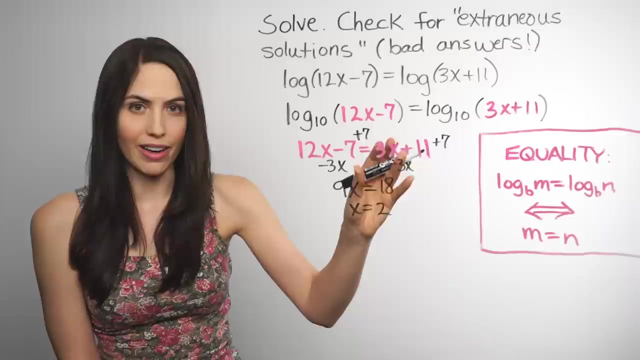 done. but with these log equations you actually have to check the numbers you get. So take the number and plug it back into the original log equation and make sure everything checks out. The reason is that sometimes the algebra you do after leaving the logs behind can magically turn up extra numbers that don't. 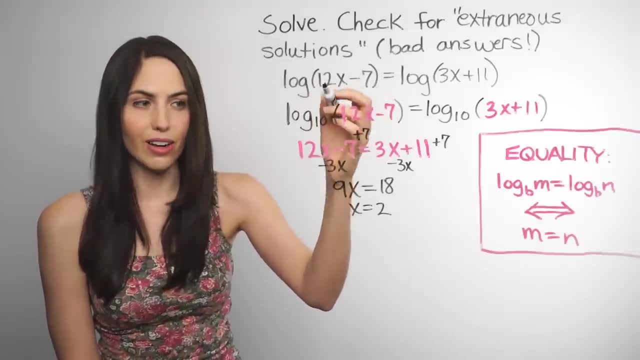 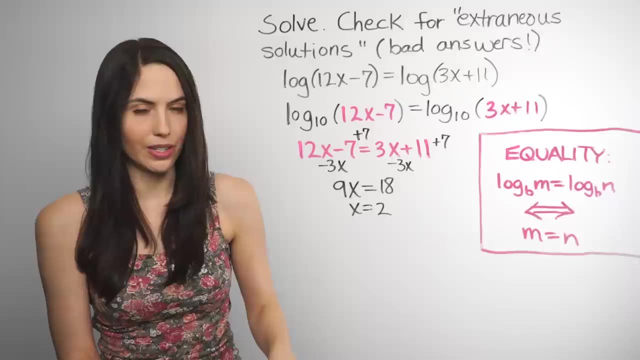 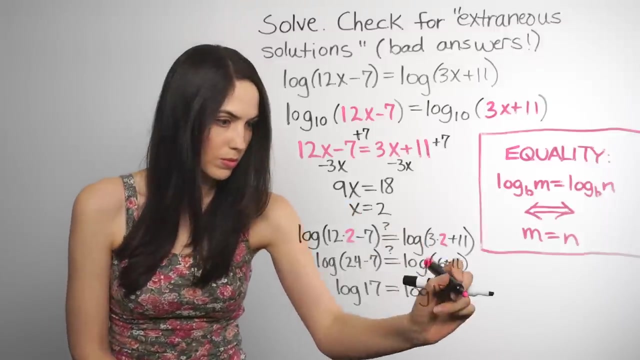 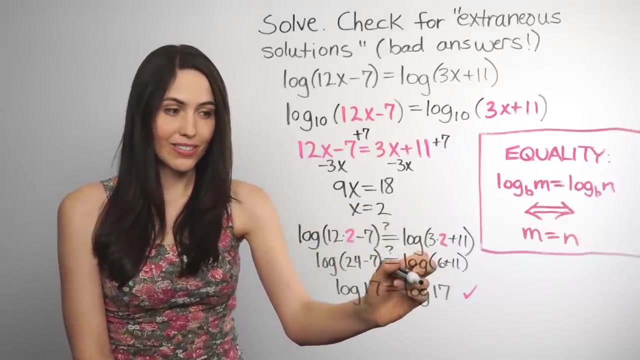 actually work for the log for the domain of the log. Let's try it. So you take that number for x and plug it in for x in the original log and make sure everything checks out Alright. when you plug in 2 for x, you end up getting log of 17 equals log of 17,. 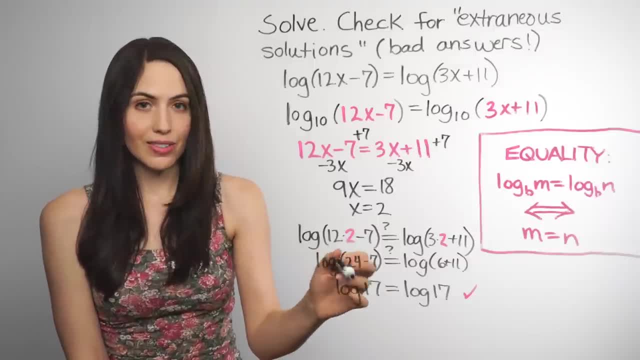 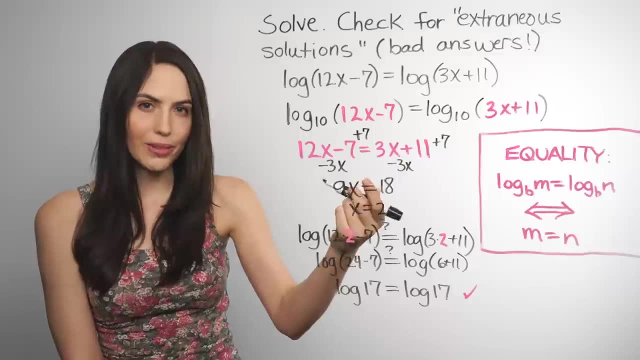 which is true. but also log of 17 is perfectly fine because you get the log of 17.. because that's in the domain of the log. By the way, if you ever got log of a negative number, you would have to throw out that answer. 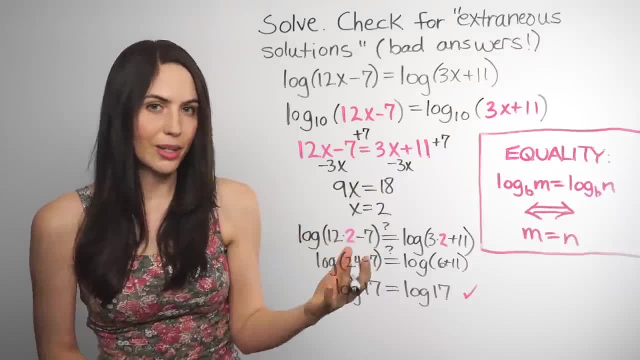 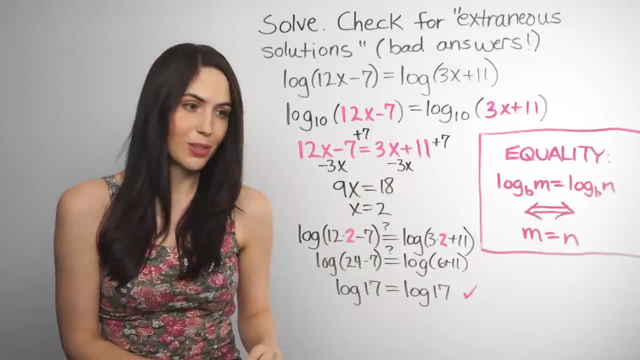 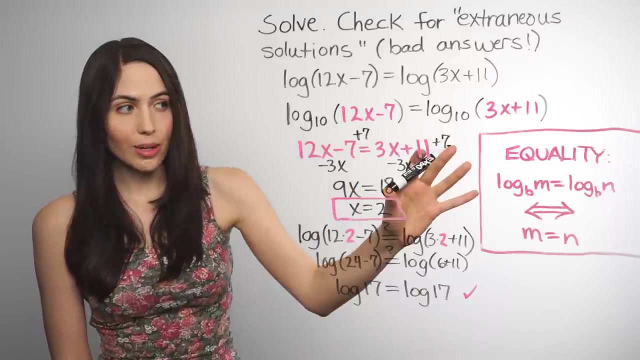 because log of a negative number is undefined in the real number system for the domain of the log. But ours is fine, R2 is fine, It checks out, so we can box that And that's our answer. So that's the equality property. 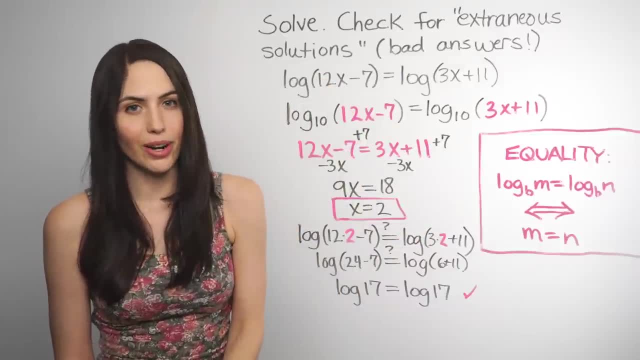 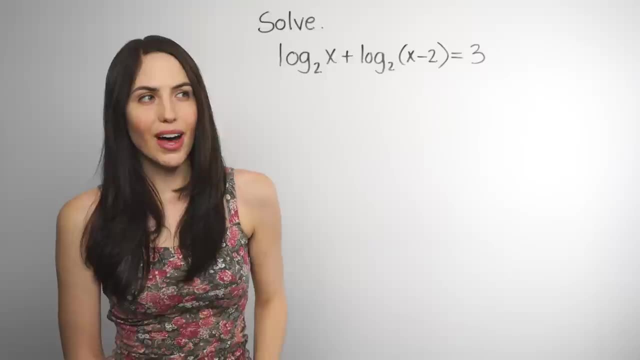 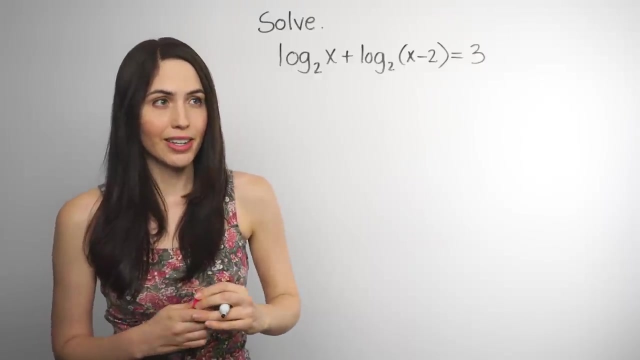 if you have one log equals another. Now let me show you the product property. All right, what if you have two logs on one side of the equation and then just a number on the other? Don't worry, You're going to use a property. 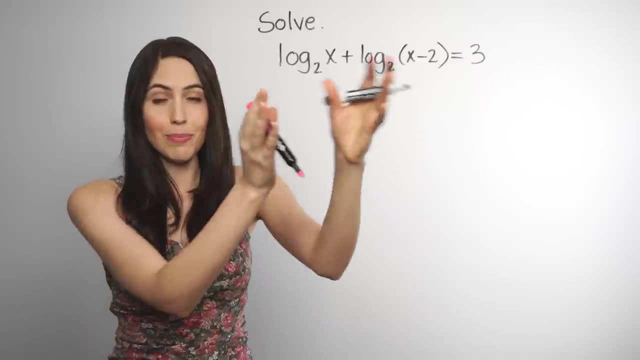 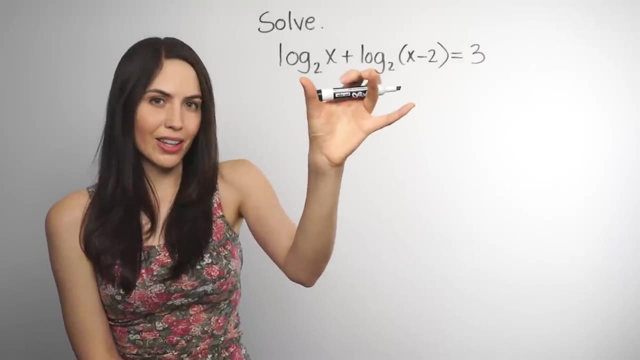 And a lot of the work of these equations is taking the multiple logs and combining them into one And with something like this, two logs added together is going to end up being the same as one log plus another log, And that's going to end up being the same as one log plus another log. 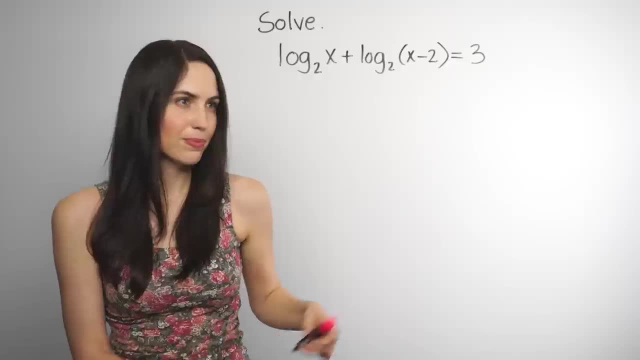 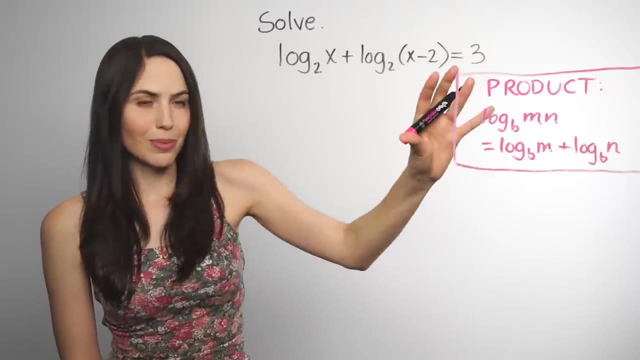 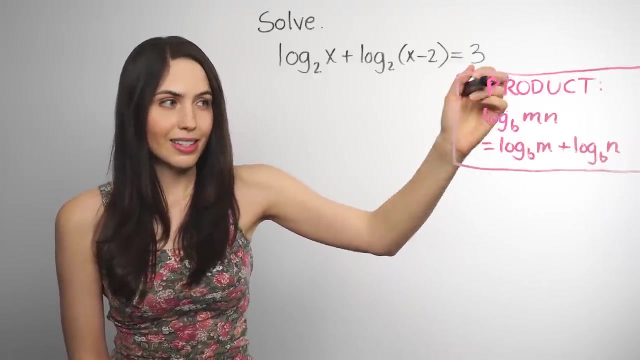 And that's going to end up being the same as one log plus another log. Let me show you what I mean. Okay, so this is the product property, And all it says is that the sum of two logs is the log of a product. 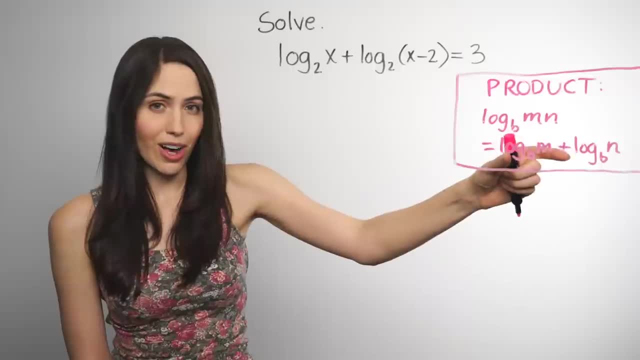 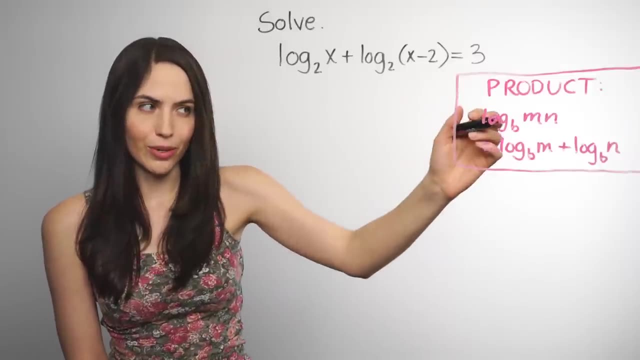 In other words, addition outside two logs is the same thing as multiplication inside a log. I'll show you what I mean. By the way, this is for variables that are positive and when the base is not equal to one. But anyway, what does that mean for us? 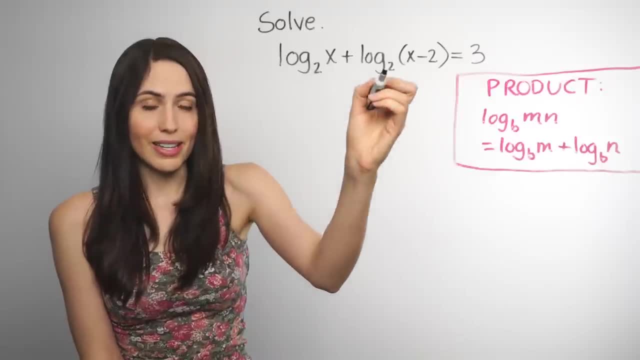 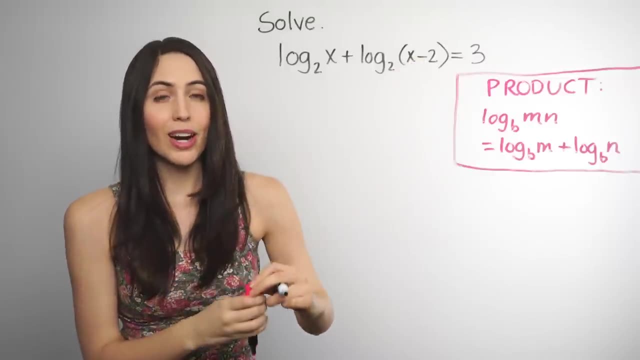 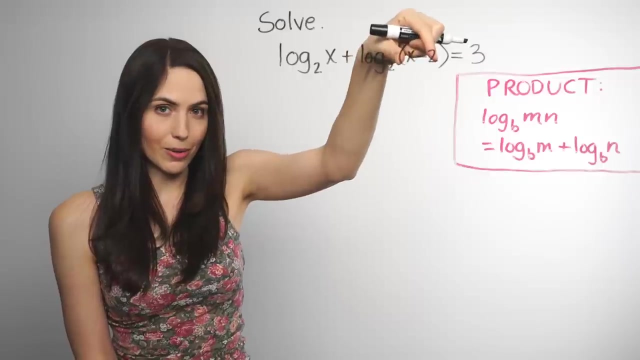 For our example, it means that because these bases are the same, both have base two, instead of having two logs added together on the left we can write it as one log of these two, multiplied One log of x times x minus two. 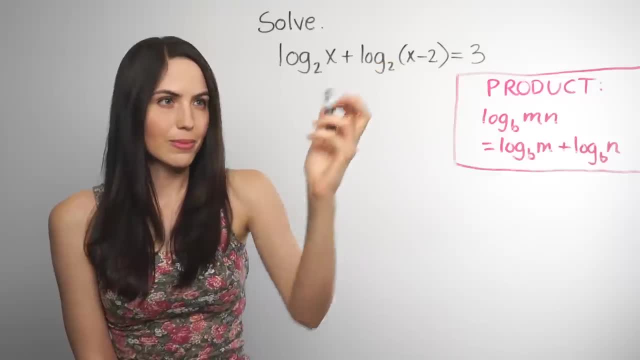 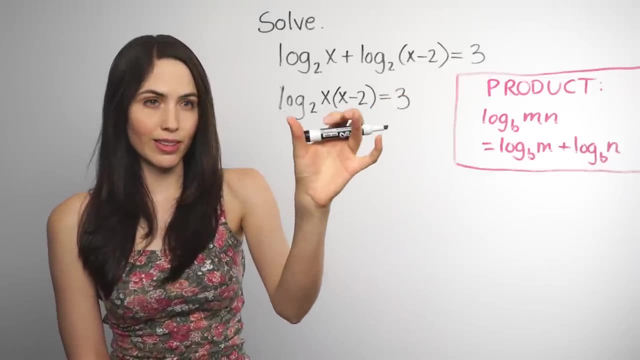 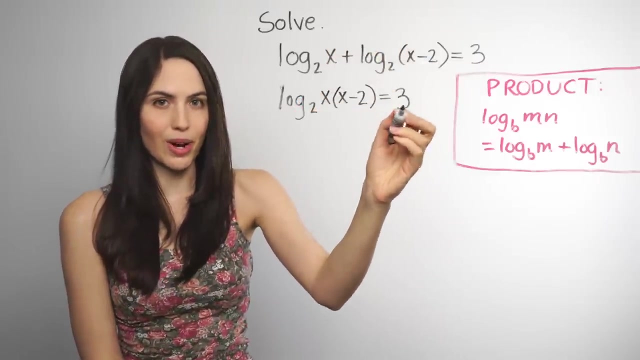 the log of their insides, their arguments multiplied All right, so we've rewritten it as one log. So we have just log base two of x times x minus two And it still equals three on the right. This is great because we just have one log in the equation now. 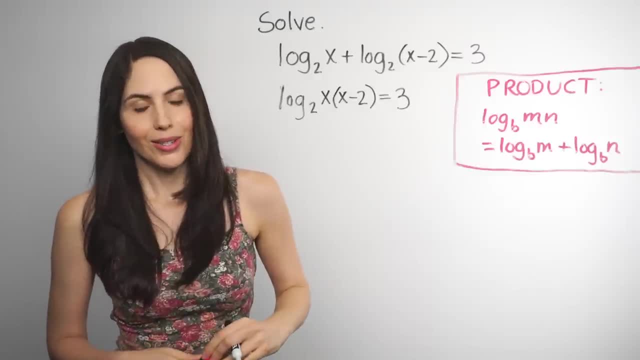 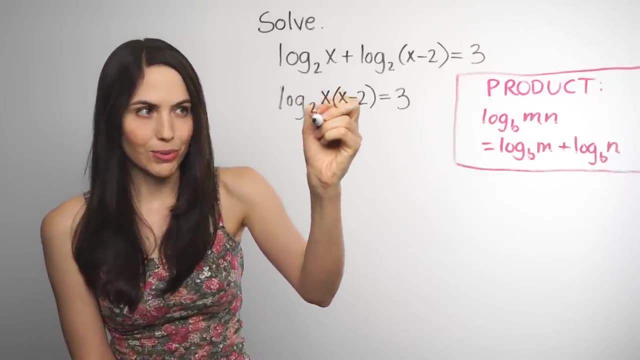 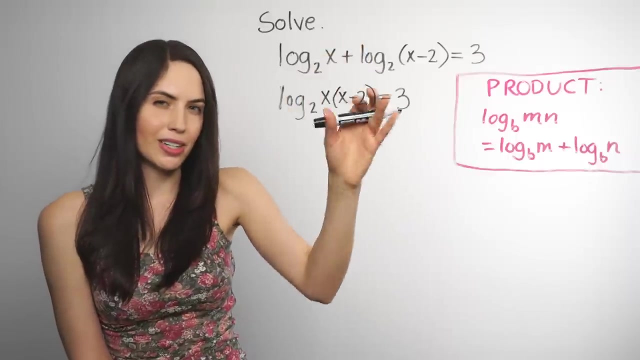 And we can use what you know from before to solve by rewriting it into exponential form. So that would look like: base two raised to the power of three Equals this part x times x minus two. That's how you rearrange it into exponential form. 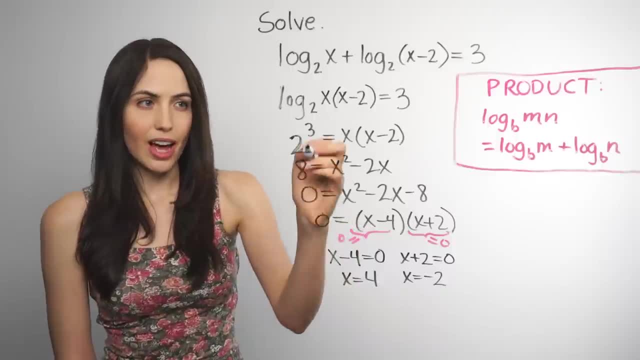 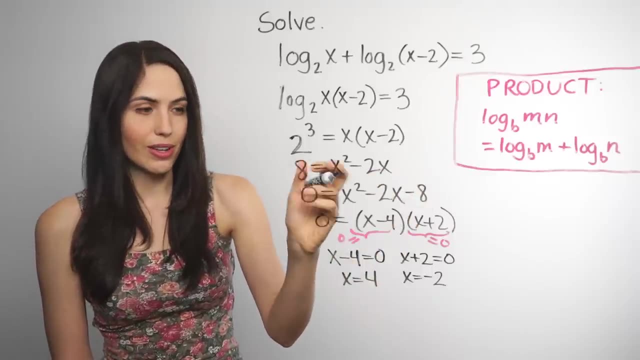 All right. so here's all the algebra we do to solve. after you write it in exponential form, You want to get everything on one side and just zero on the other side so that you can solve. And this quadratic you can factor into x minus four, x plus two. 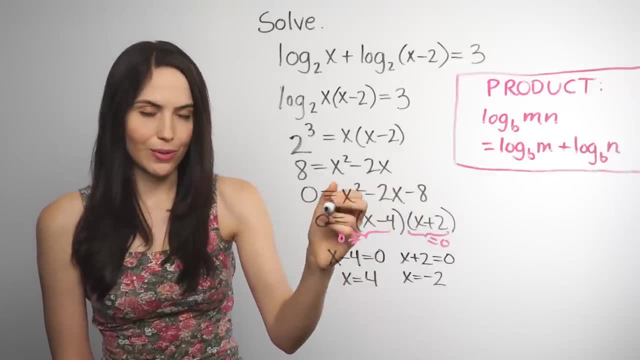 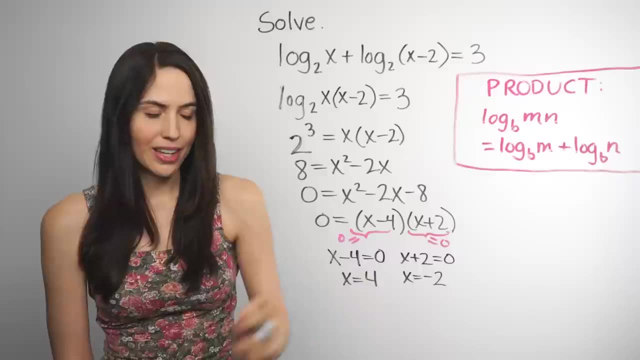 And once you have it in factored form, x equals zero. The way you solve is setting each factor equal to zero And we get x equals four and x equals negative two. It's tempting to think that you're done, I know. 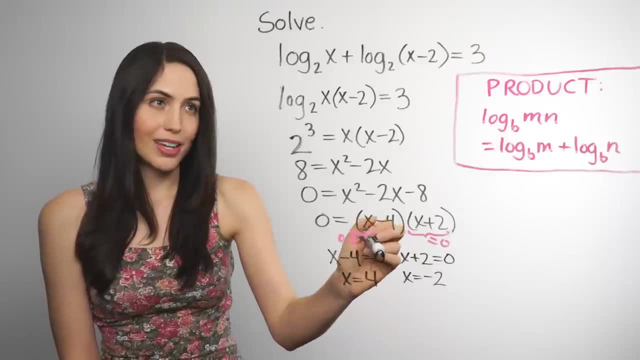 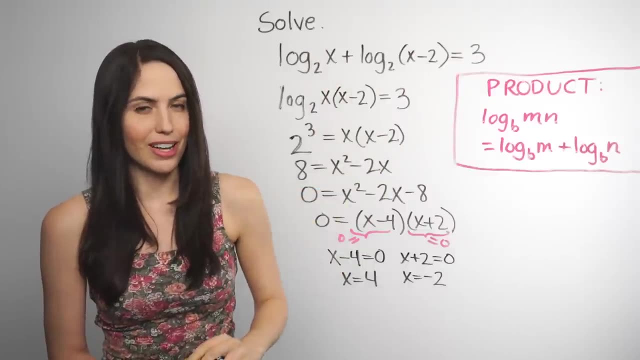 But again we have to take those numbers and check them in the original equation- And I know, I know I didn't write check your solutions this time. I left it out on purpose because your teachers will do that sometimes to really test you. 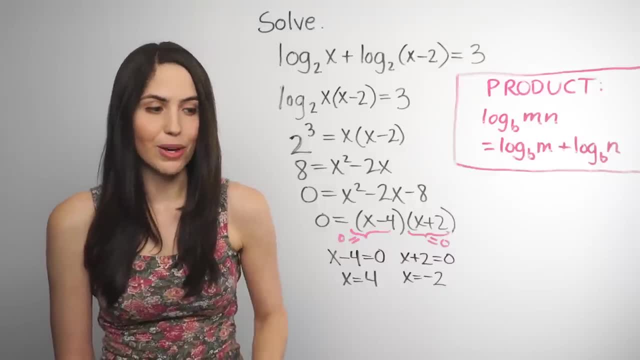 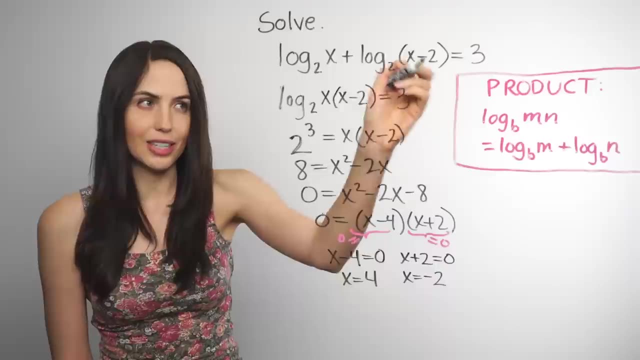 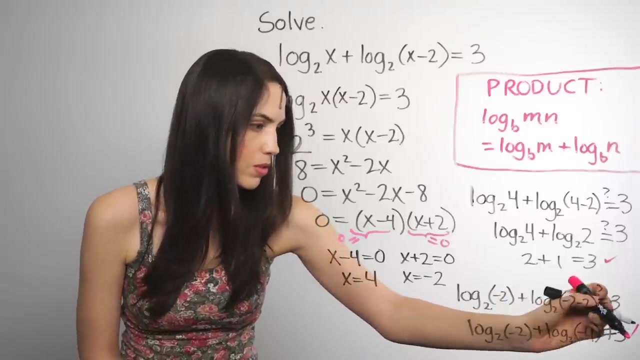 They're trying to trick you. It's shady, I know, But we have to check those numbers. So we'll take four and negative two and plug them each in for x in the original equation. All right, so we check both answers. 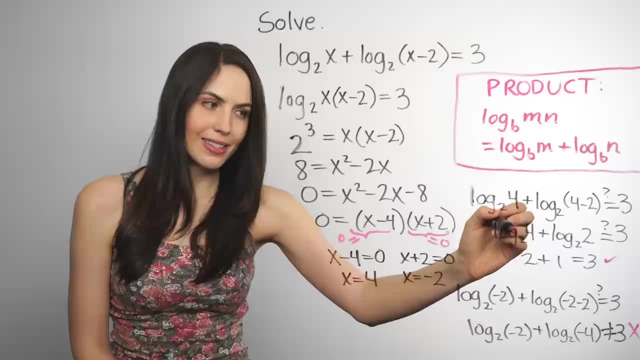 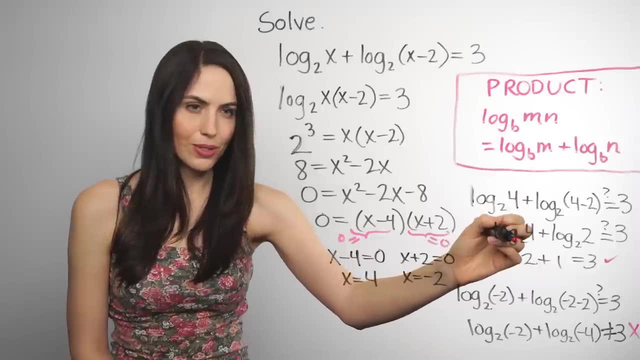 When we check four for x, you end up getting this Log base. two of four is just two. because two to the two powers four, That's just equal to two. This is just equal to one, because two to the one powers two. Anyway, on the left side, 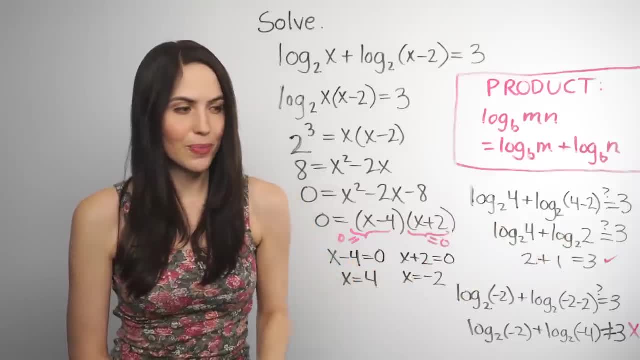 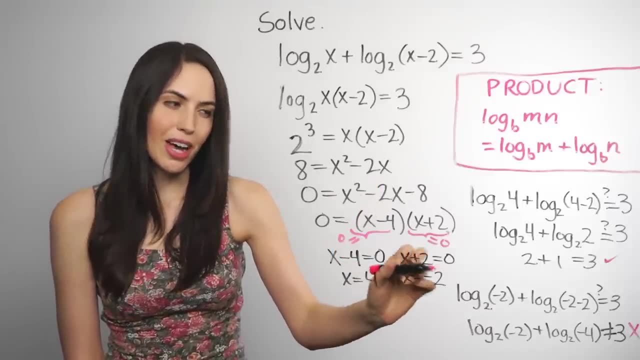 it's really two plus one, which is equal to three. So that checks out And that means that four is an actual answer. Now, negative two. when we check that one, we end up getting logs of negative numbers, And any time you get a log of a negative number. 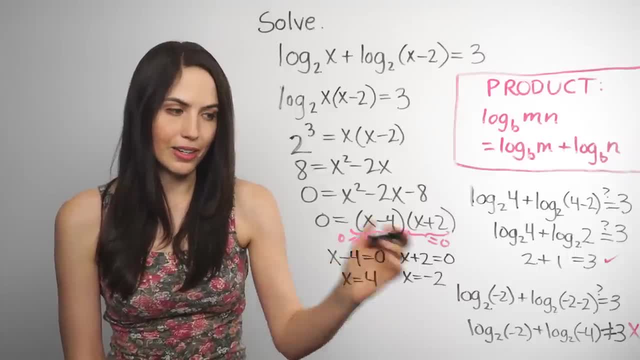 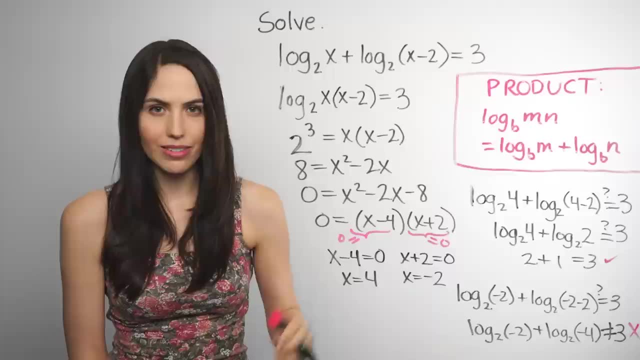 it's undefined in the real number system. The negative number is not in the domain of the logs, So whatever caused that to happen has to be thrown out as an answer. So it's not really an answer And the only actual answer is: x equals four. 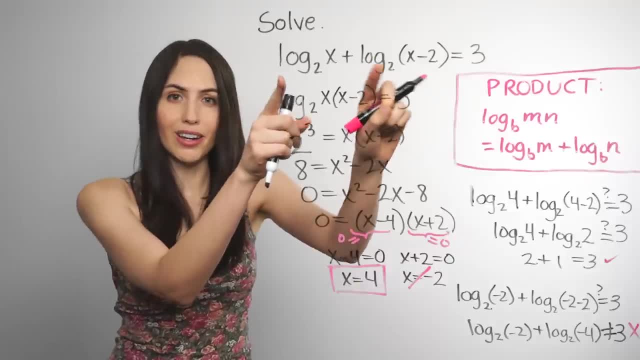 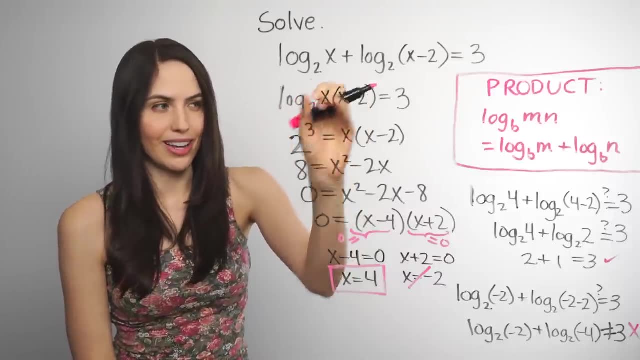 So that's how you use the product property. if you have two separate logs added and they have the same base, You can put them together as one log of the two insides multiplied. Now let me show you an even more complicated equation where you need the quotient property. 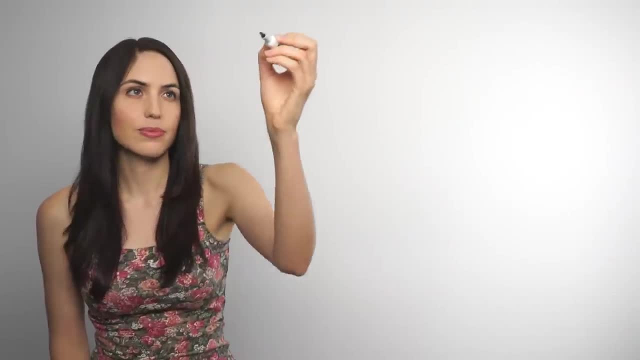 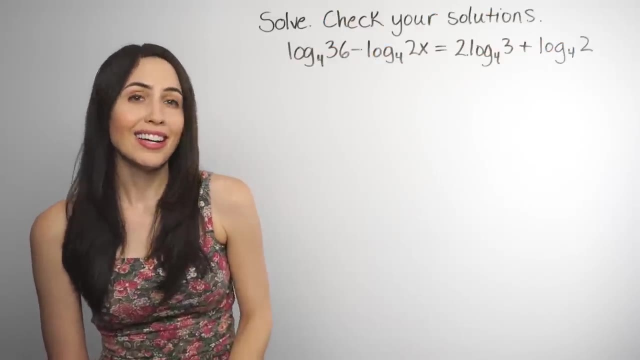 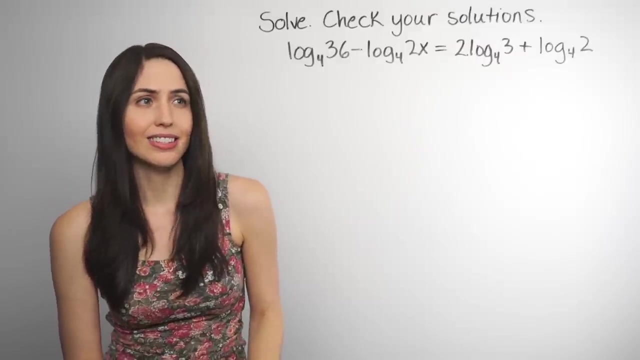 and the power property. Oh, but it gets better, guys. Now we have four logs and one of them has a number multiplied in the front. What a mess. Yeah, you can't unsee that, But it's actually not that bad. 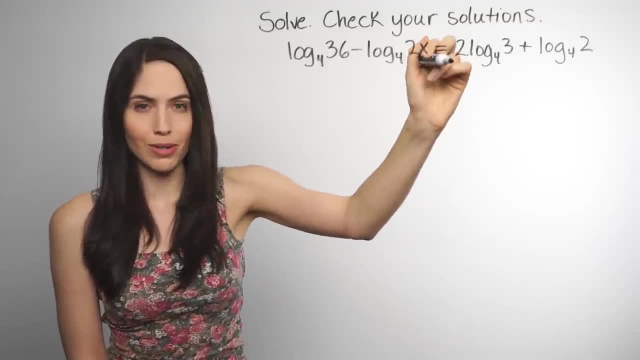 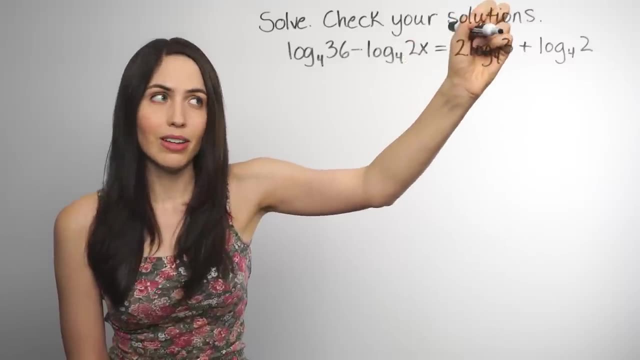 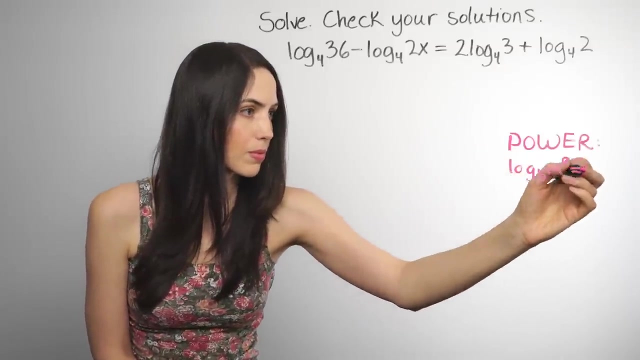 because the first thing you want to do is, any time you do see one of those numbers multiplied in front of a log, you use this new property, the power property, and you bring it up as a power inside the log. Okay, so this is the power property. 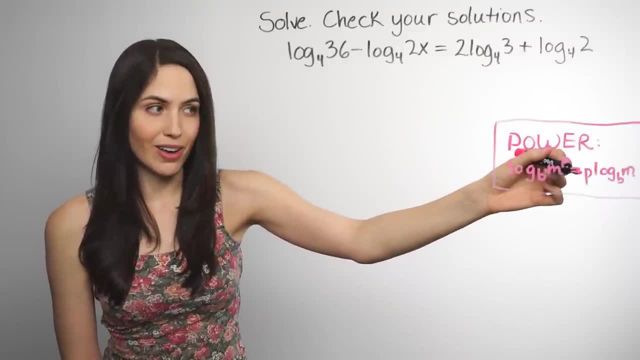 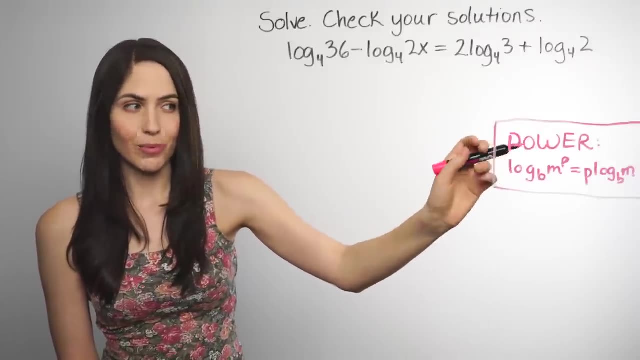 and all it says is that if you have a number multiplied in front of a log, you can bring it up as a power inside the log, And this is true for real powers, p and when m and b are positive and b not equal to one. 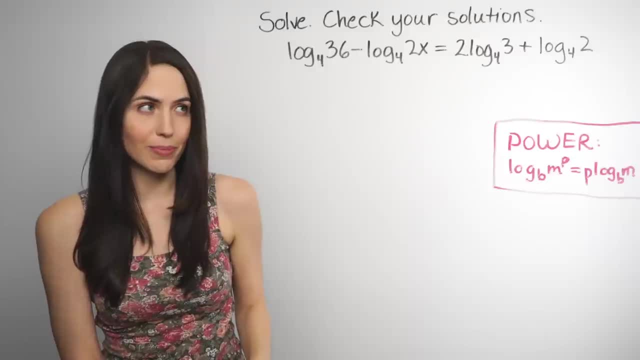 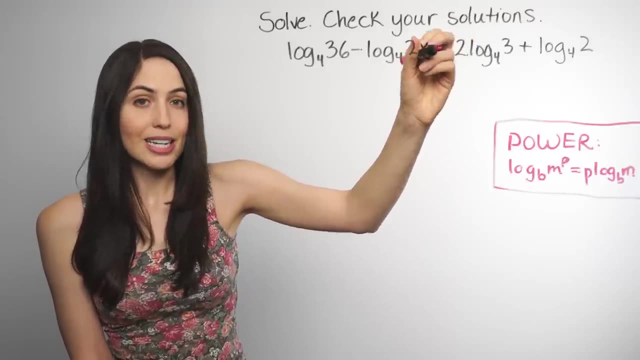 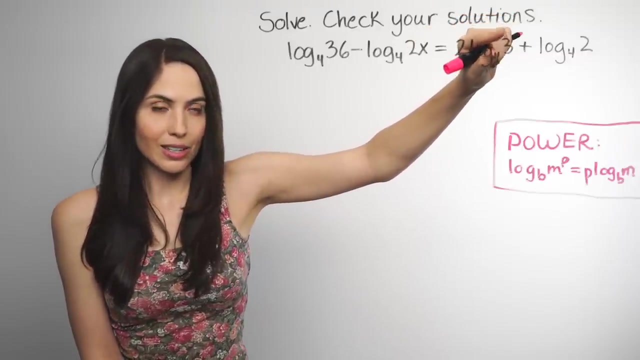 That's my disclaimer. But anyway, for our problem, because we have this number multiplied in front the two as a coefficient, we can use the power property and bring that two up as a power here for the three inside the log. So this term will become log base four. 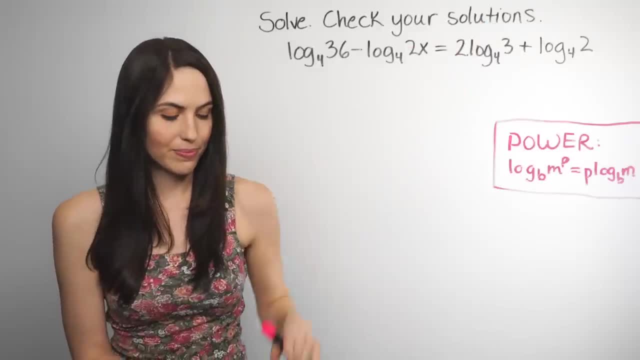 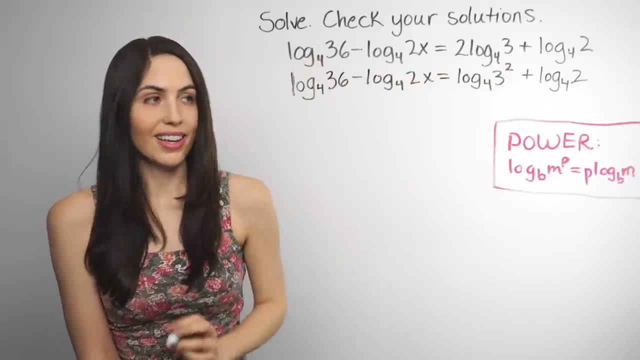 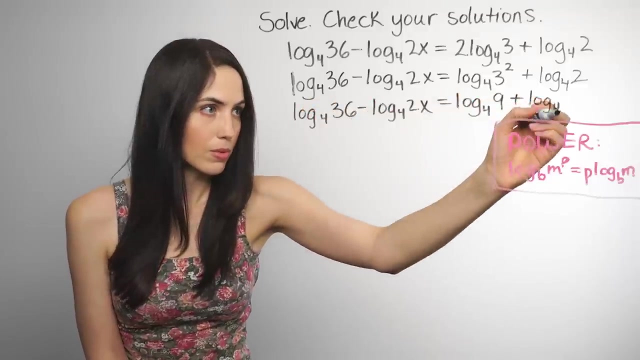 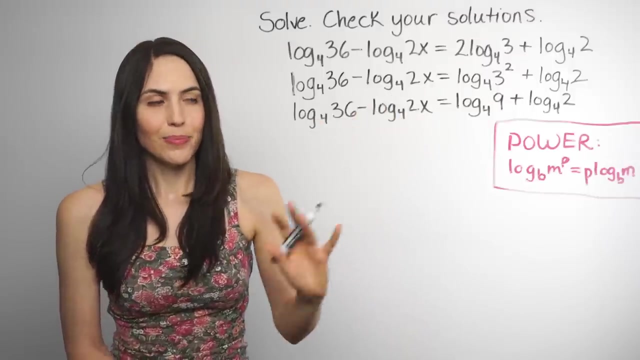 of three to the two power three squared, And of course, three squared is just nine, so we can replace that with nine. Okay, now it's starting to look more like something we've seen before. kind of Try to use what you already know. 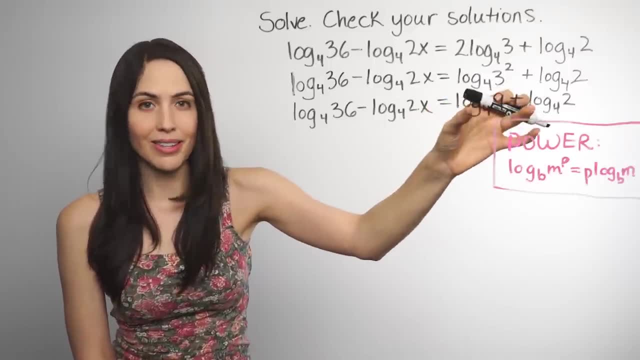 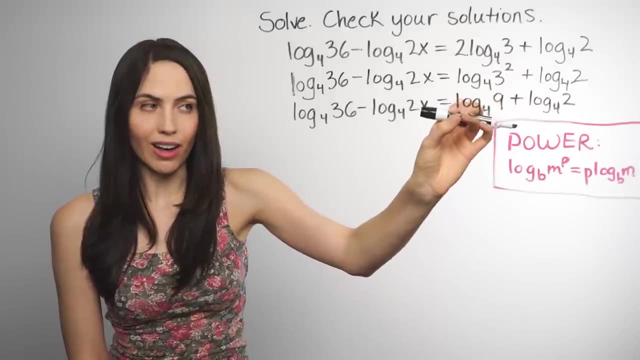 and if you see two logs added together and they have the same base, think of that property from before, the product property, where you can combine them into one, one log, that is, of the product of these two. So log base four of nine times two. 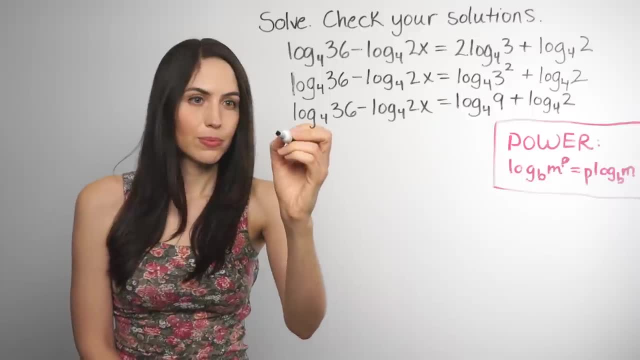 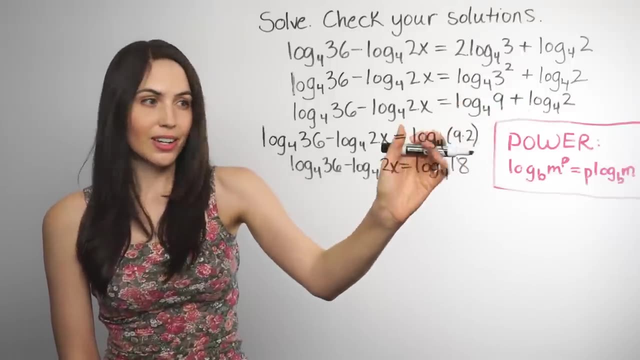 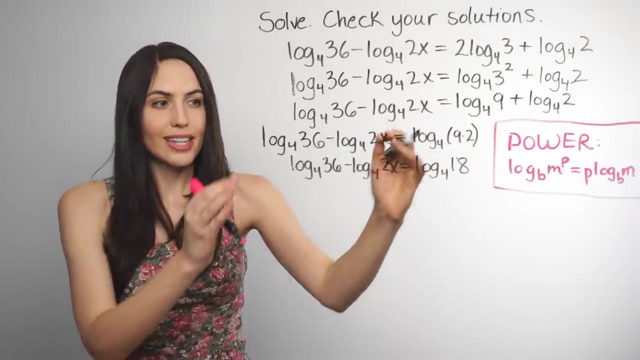 combined into one log. So we combine those two logs together became log base four of nine times two, which is a log base four of 18.. And this is our current version of the log equation. It's getting more and more simple. 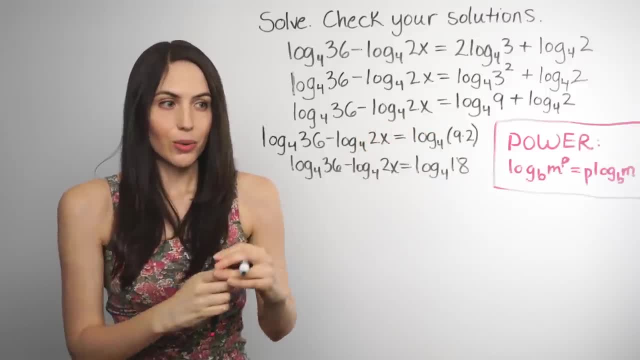 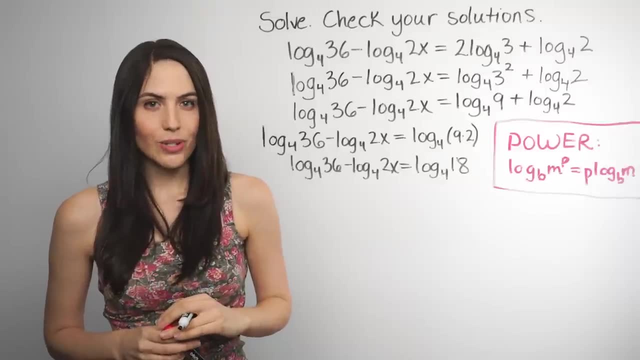 more and more condensed, as they say. which is what you want Really? we want just one log on each side, max. So now, looking at this, there's not much more you can do on the right, but on the left. 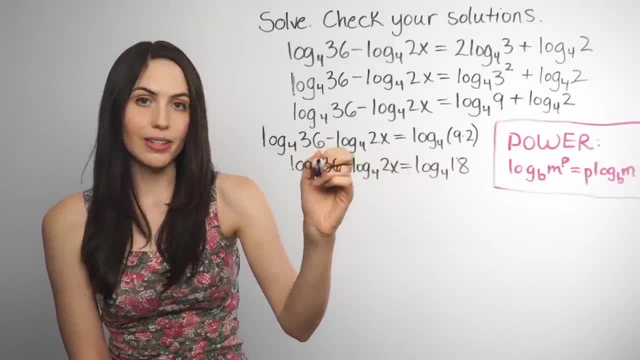 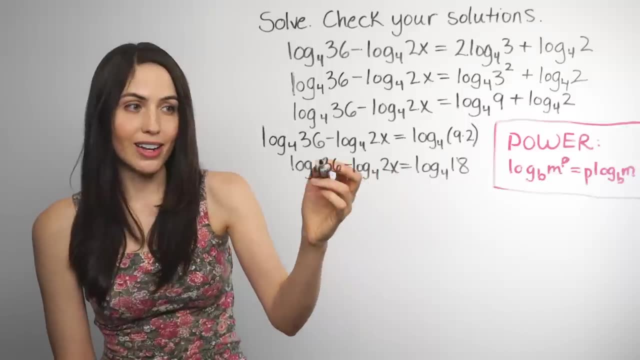 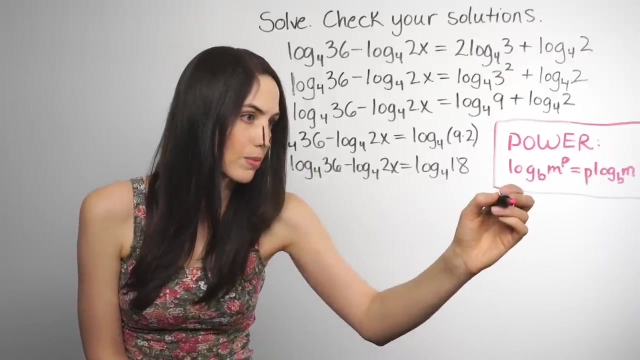 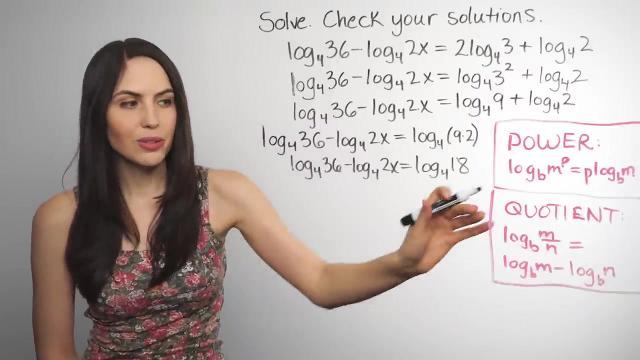 you may already have guessed this, but when you have two logs subtracted, one log minus another and they have the same base, there's a property for that, And it's not the product property but the quotient property. So this is the quotient property. 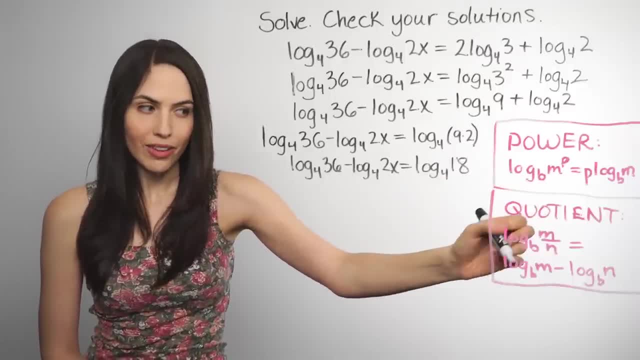 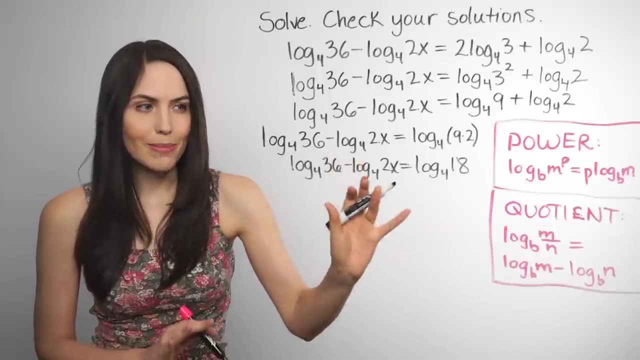 and all it says is that if you have one log subtracted from another and they have the same base, you can rewrite it as a single log of one inside over the other inside. What that means for our problem is that on the left side,